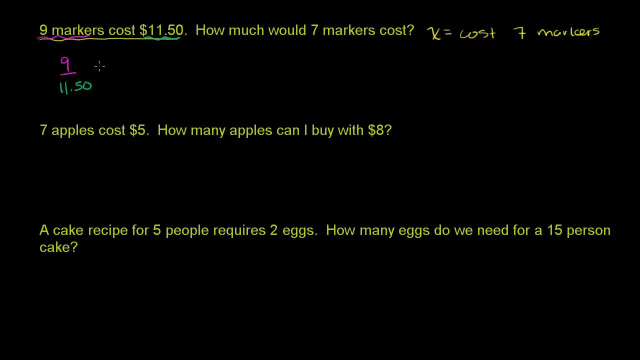 to $11.50,. this should be equal to the ratio of our new number of markers. 7, equal to the new number of markers. So that's 7.. To whatever the new cost or whatever the cost of the seven markers are. 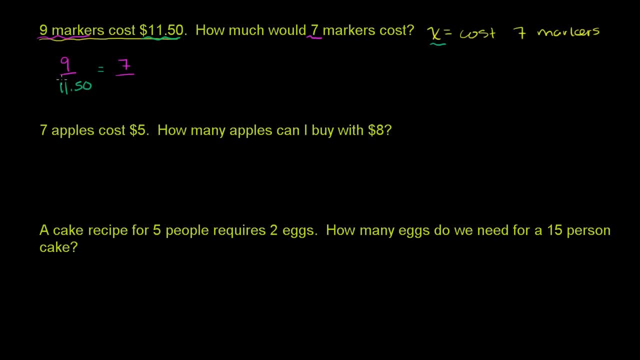 To x. So let me do x in green To 2x. So this is a completely valid proportion. here. The ratio of nine markers to the cost of nine markers is equal to seven markers to the cost of seven markers. And then you could solve this to figure out. 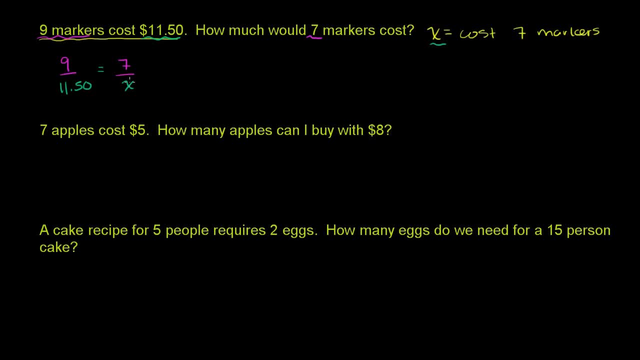 how much those seven markers would cost. And you could flip both sides of this and it would still be a completely valid ratio. You could have $11.50.. $11.50 to $9.00.. So the ratio between the cost of the markers. 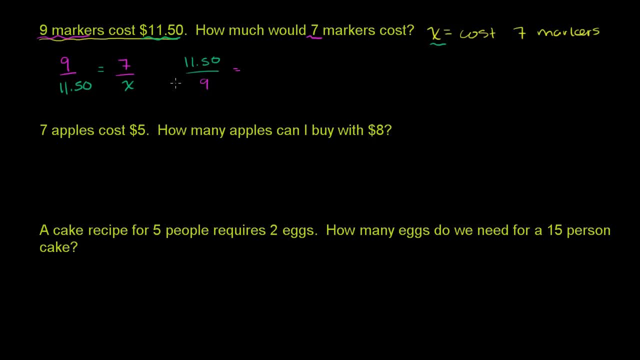 to the number of markers you're buying is equal to. so $11.50 to $9.00 is equal to the cost of seven markers, is equal to the ratio of the cost of seven markers to the number of markers, which is obviously seven. 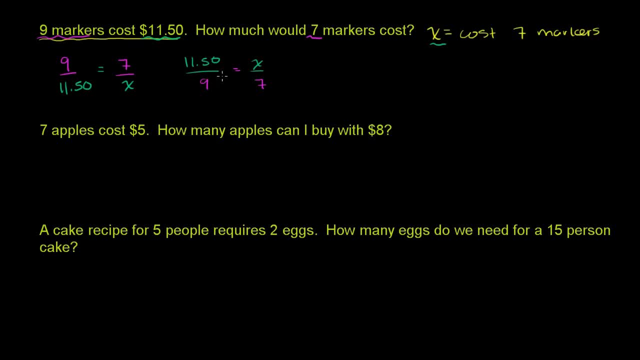 So all I would do is flip both sides of this equation right here to get this one over here. You could also think about. you could also think about the ratios in other ways. You could say that the ratio of nine markers to seven markers is going to be the same as the ratio of their cost. 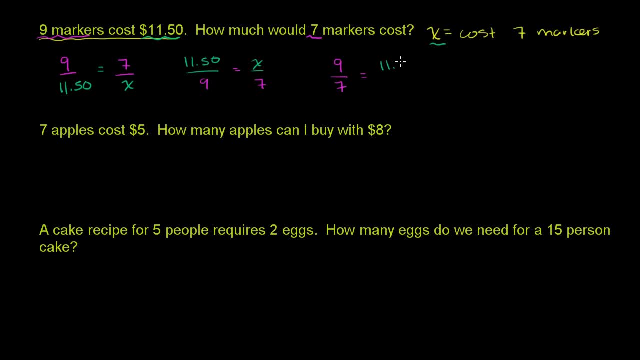 is going to be equal to the ratio of the cost of nine markers to the cost of seven markers. And then obviously you could flip both of these sides So you could say that the ratio of seven markers. maybe that's the same magenta color. 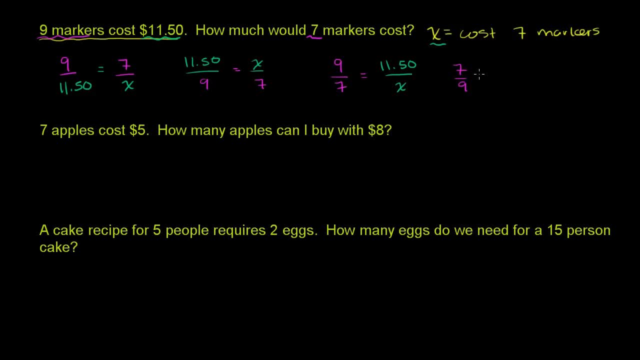 the ratio of seven markers to nine markers is the same thing as the ratio of the cost of seven markers to the cost of nine markers. So that is $11.50.. So all of these would be valid proportions, valid equations that describe what's going on here. 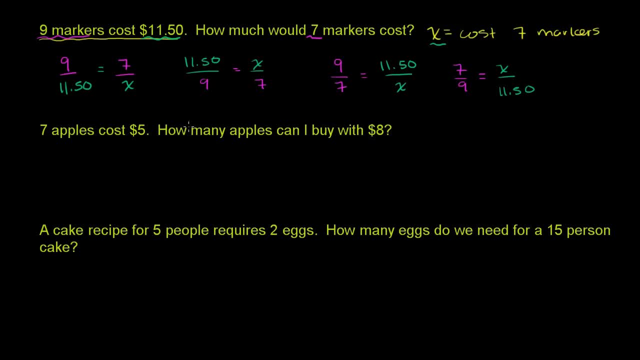 And then you would just have to essentially solve for x. So let's do this one right over here: Seven apples cost $5.00.. How many apples can I buy with $8.00?? So once again we can say: so, we're. 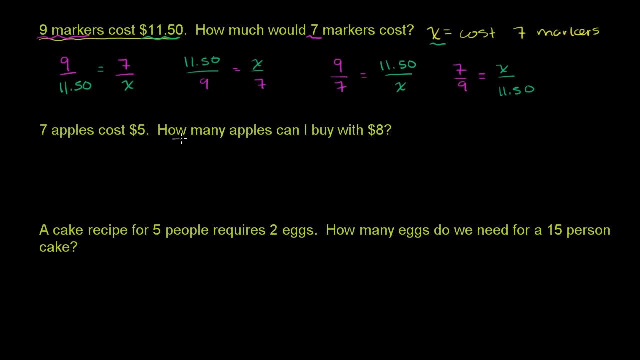 going to assume that what they're asking is how many apples. let's call that x. x is what we want to solve for. So seven apples cost $5.00.. So we have the ratio between the number of apples seven and the cost of the apples five. 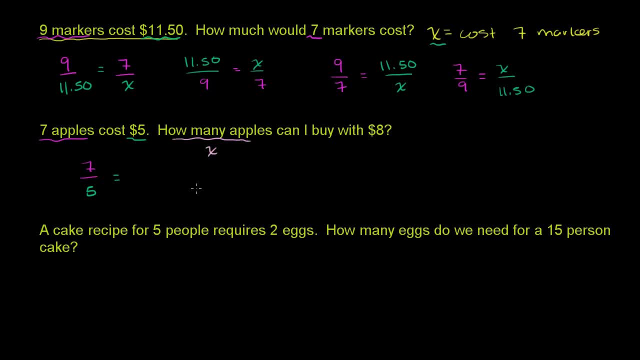 is going to be equal to the ratio between another number of apples, which is now x, and the cost of that other number of apples, And it's going to be $8.00.. And so notice here, in this first situation, what was unknown was the cost. 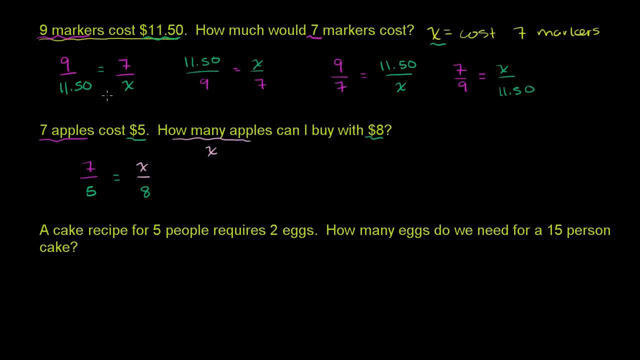 So we kind of had the number of apples to cost, number of apples to cost. Now, in this example, the unknown is the number of apples, So number of apples to cost, number of apples to cost. Now we could do all of the different scenarios like this. 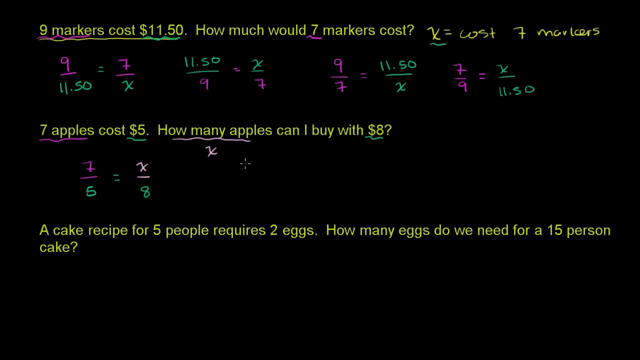 You could also say the ratio between seven apples and x apples is going to be the same as the ratio between the cost of the apples, The cost of seven apples and the cost of eight apples. And obviously you could flip both sides of either of these equations to get two more equations. 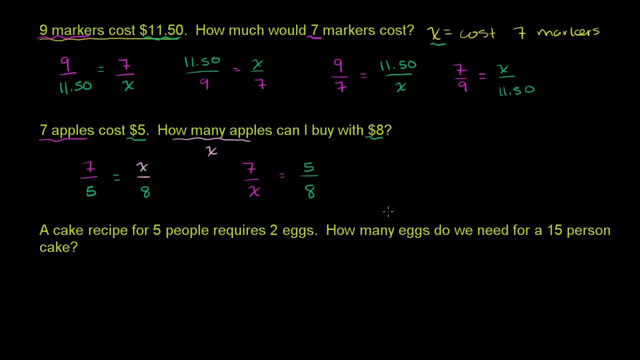 And any of these would be valid equations. Now let's do this last one. So we have a cake recipe for five people. I'll use new colors here. A cake recipe for five people requires two eggs. It requires two eggs. How many eggs? 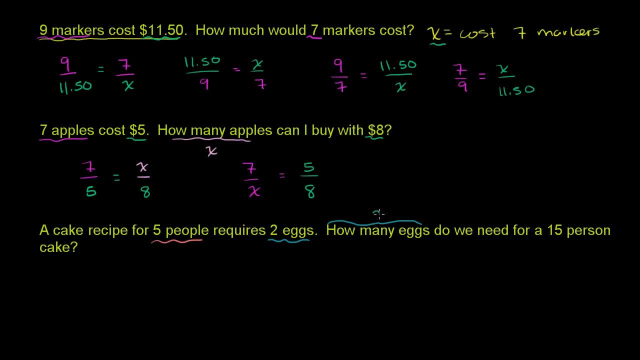 So we want to know how many eggs. So this we'll call x, And you don't always have to call it x. You could call it e for a. Well, e isn't a good idea because e represents another number once you get to higher mathematics. 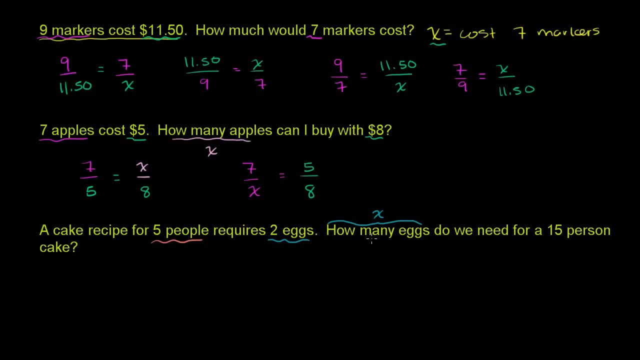 But you could call them y or z or any variable, a, b or c, anything. How many eggs do we need for a 15-person cake? How many eggs do we need for a 15-person cake? So you could say the ratio of people to eggs is constant. 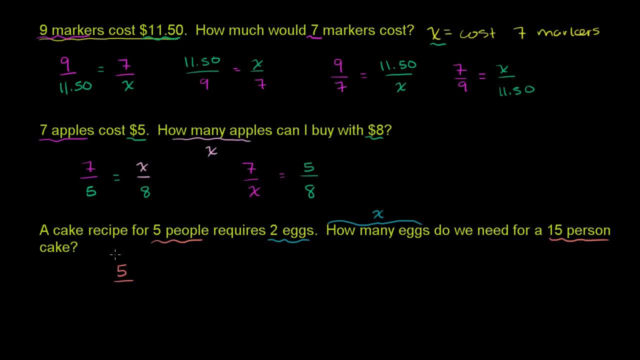 So if we have five people for two eggs, then for 15 people we are going to need x eggs. This ratio is going to be constant. 5 over 2 is equal to 15 over x, Or you could flip both sides of this.